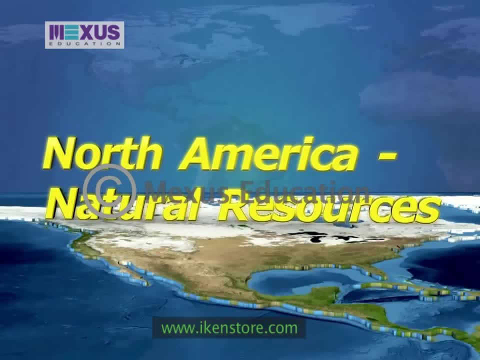 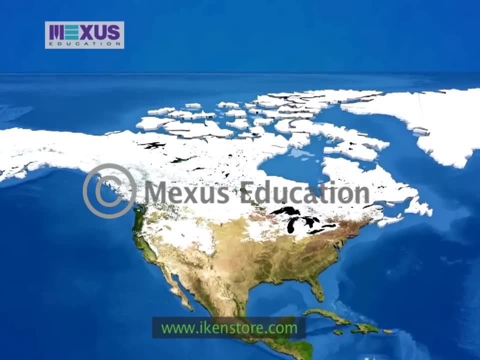 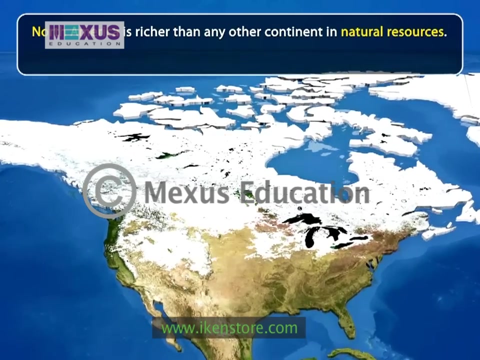 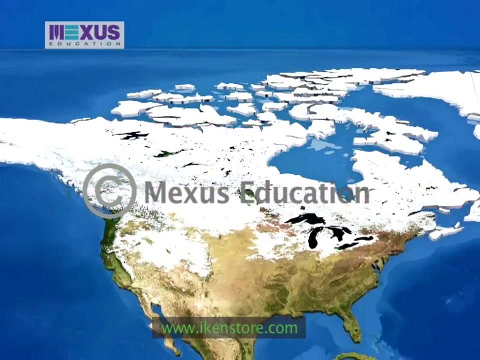 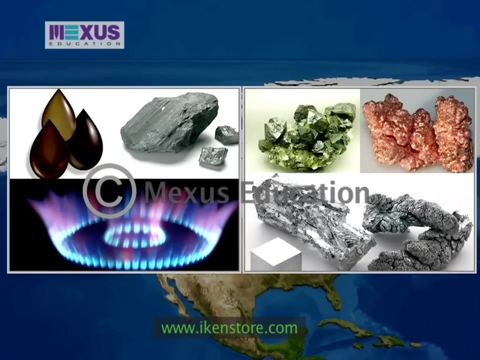 North America is richer than any other continent in natural resources. This has made USA and Canada two of the most advanced and modern countries in the world. North America is very rich in minerals, especially fossil fuels and metallic minerals, which form the base of modern industry. 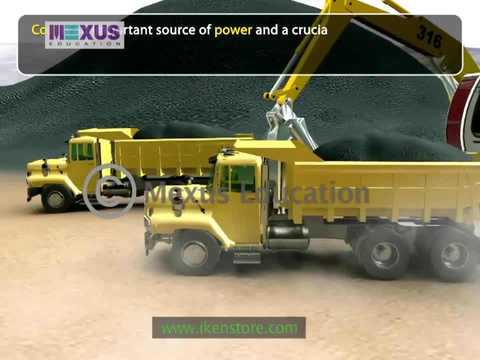 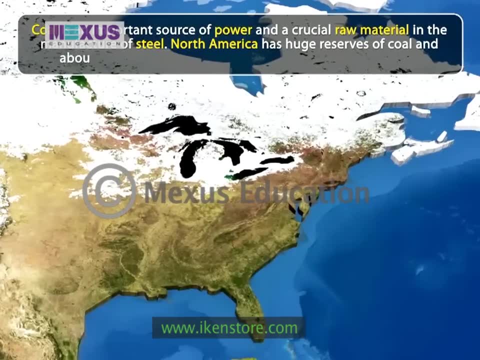 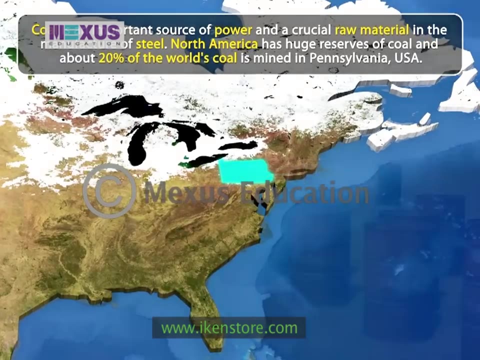 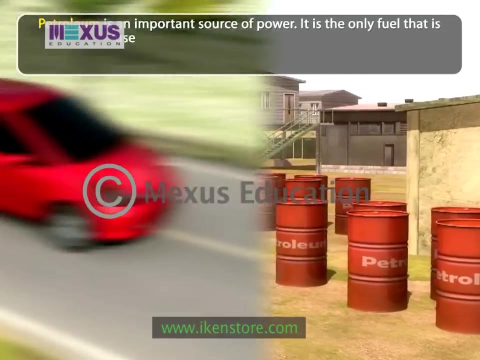 Coal is an important source of power and a crucial raw material in the manufacture of steel. North America has huge reserves of coal and about 20% of the world's coal is mined in Pennsylvania, USA. Petroleum is an important source of power. It is the only fuel that is used by modern means of transportation. 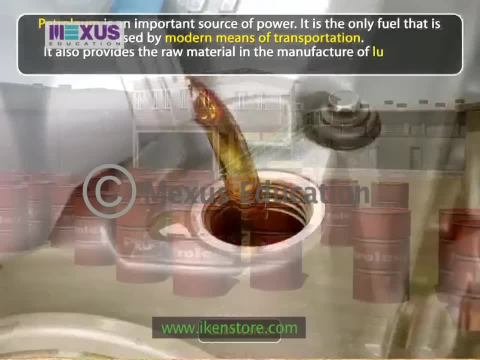 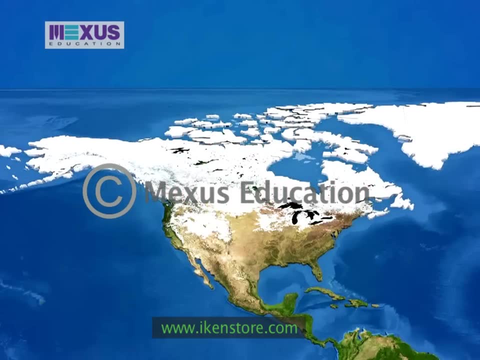 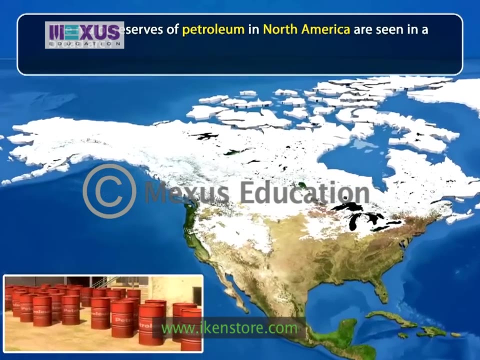 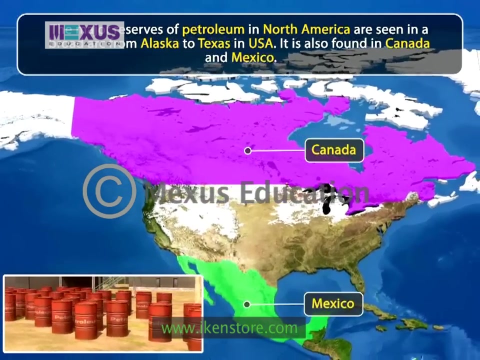 It also provides the raw material in the manufacture of lubricants, Vaseline, soap and many other products. The major reserves of petroleum in North America are seen in a broad arc from Alaska to Texas. It is also found in Canada and Mexico. USA is the third largest producer of petroleum in the world. 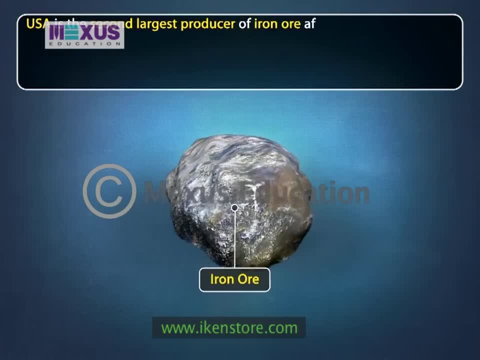 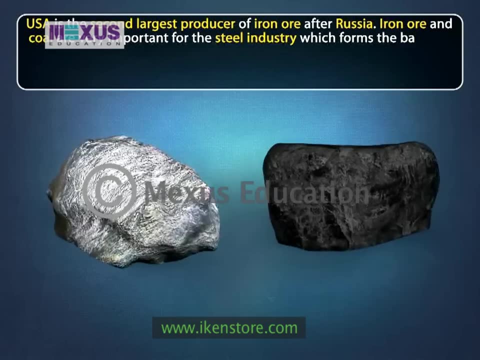 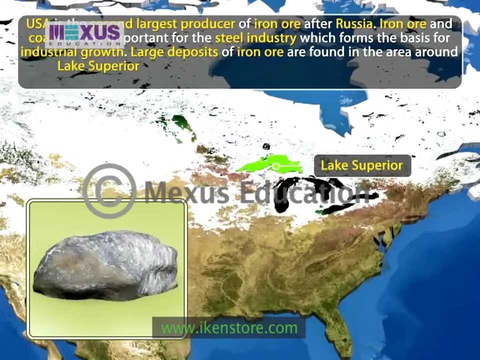 USA is the second largest producer of iron ore after Russia. Iron ore and coal are very important for the steel industry, which forms the basis for industrial growth. Large deposits of iron ore are found in the area around Lake Superior and in the eastern part of the Canadian Shield. 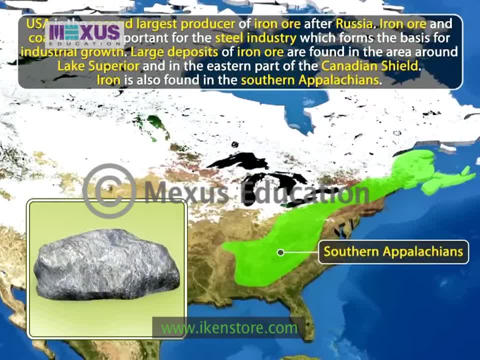 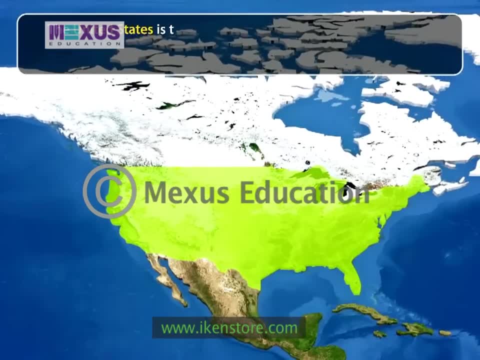 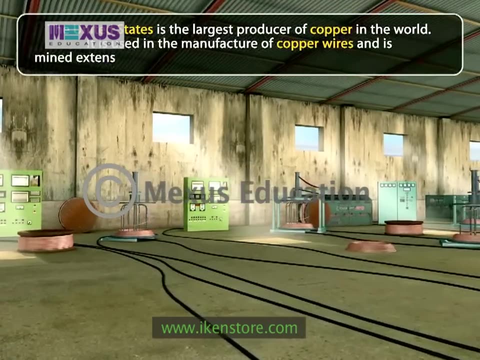 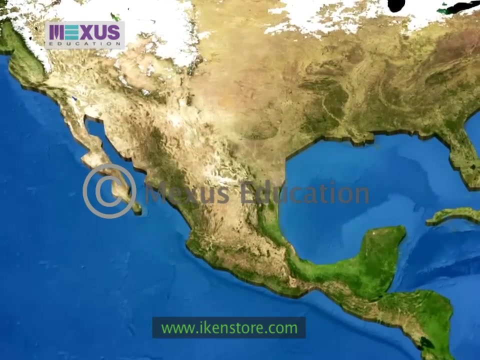 Iron is also found in the southern Appalachians. The United States is the largest producer of copper in the world. It is used in the manufacture of copper wires and is mined extensively around the Great Lakes and the Rocky Mountains. Mexico is the world's largest producer of silver. 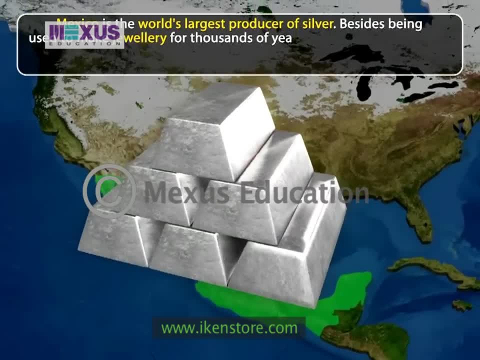 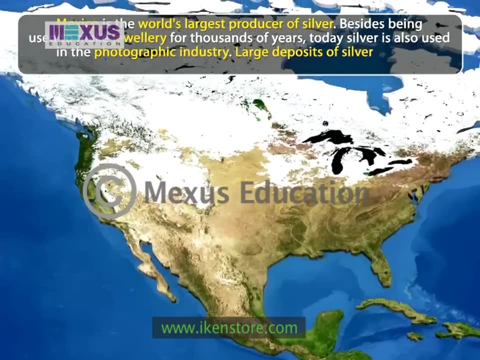 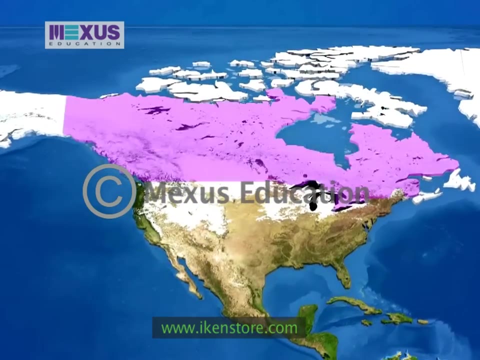 Besides being used to make jewelry for thousands of years, today silver is also used in the photographic industry. Large deposits of silver are found in USA and Canada. Canada and the United States produce substantial amounts of gold, which is mined in the Rocky Mountains. 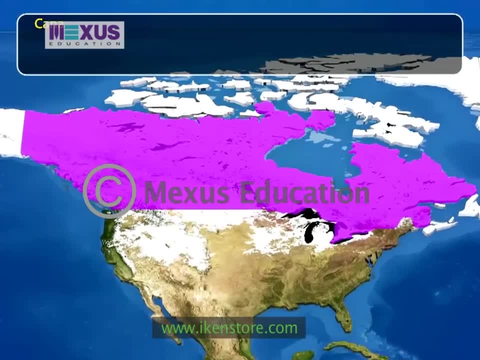 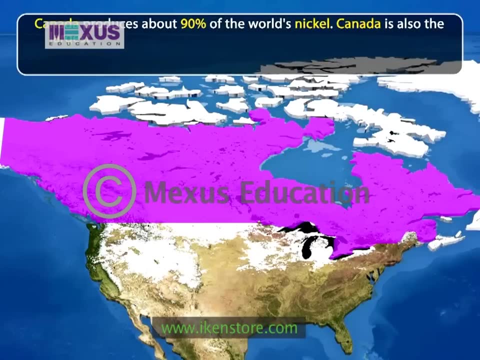 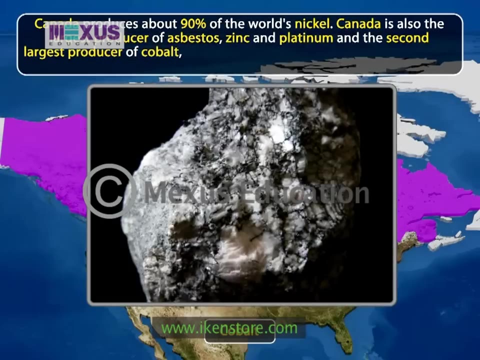 Mexico is the world's largest producer of silver. Mexico is the world's largest producer of silver. Mexico is the world's largest producer of silver. Canada produces about 90% of the world's nickel. Canada is also the largest producer of asbestos, zinc and platinum and the second largest producer of cobalt, uranium and radium. 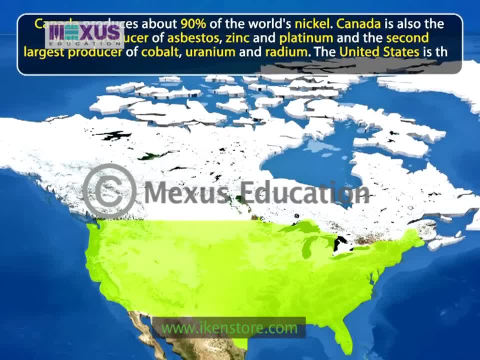 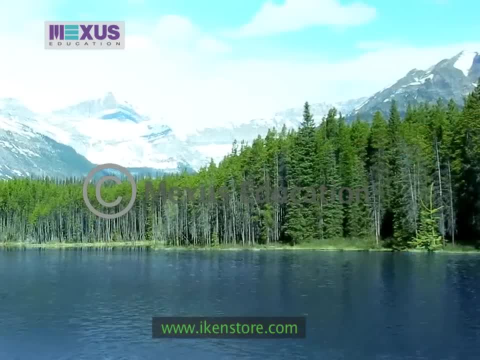 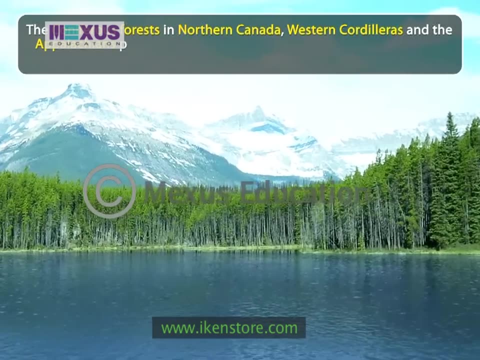 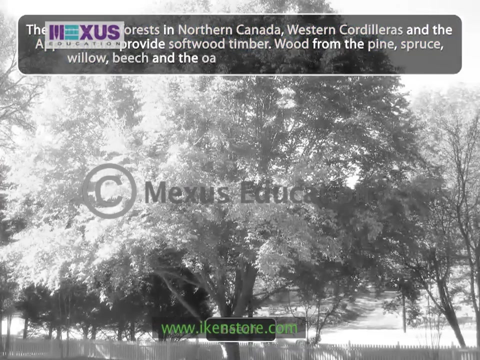 The United States is the world's largest producer of uranium and sulfur. The United States is the world's largest producer of uranium and sulfur. The coniferous forests in Northern Canada, Western Cordilleras and the Appalachians provide softwood timber. Wood from the pine, spruce, willow, beech and the oak trees is used to make furniture. 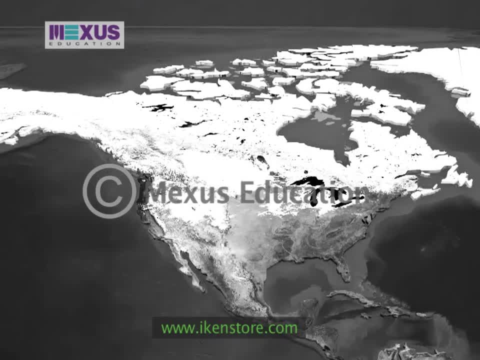 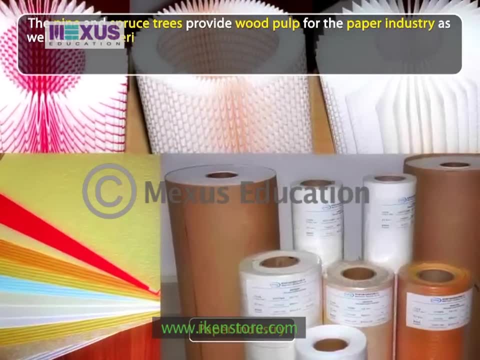 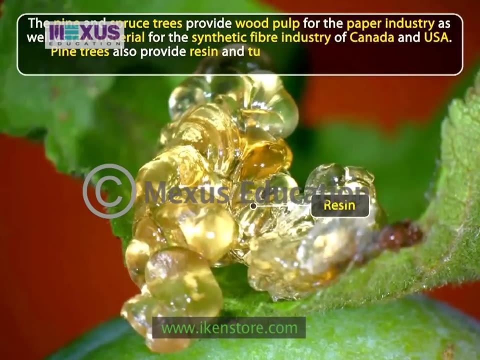 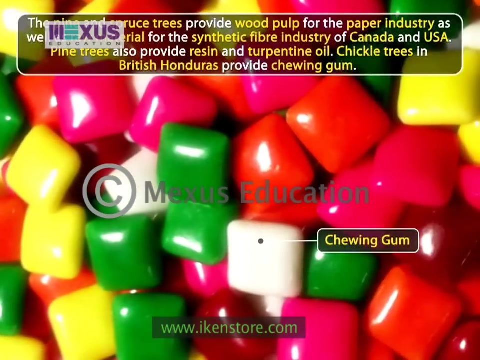 The pine and spruce trees provide wood pulp for the paper industry, as well as raw material for the synthetic fiber industry of Canada and USA. Pine trees also provide resin and turpentine oil. Chickle trees in British Honduras provide chewing gum. The tropical forests in Northern Canada are used to make furniture. 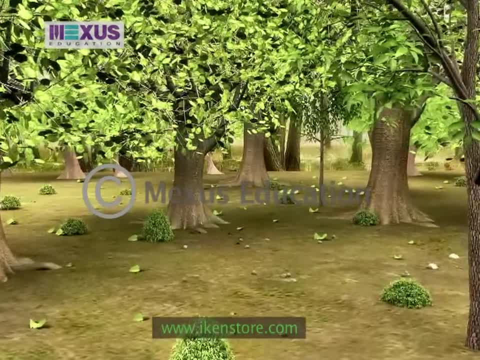 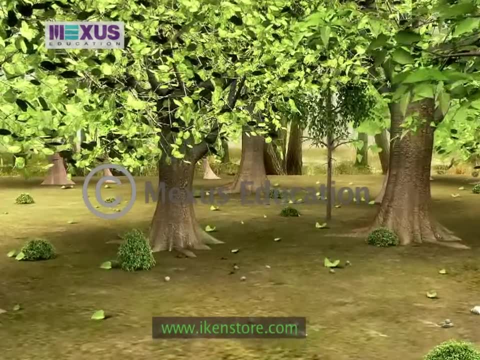 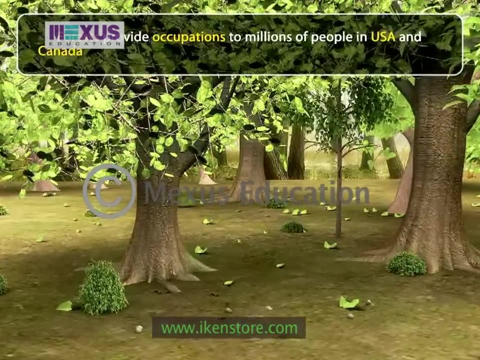 Forests provide a significant amount of timber for the manufacture of furniture and newsprint, despite being cut down to provide land for human settlement and cultivation in the past decade. Forests provide occupations to millions of people in USA and Canada in the lumbering paper, rayon and other related industries. 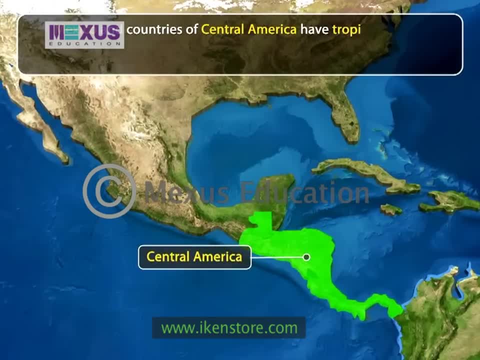 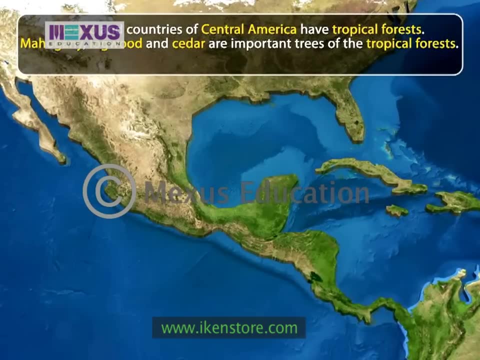 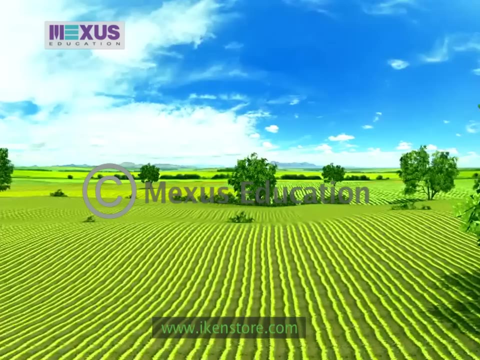 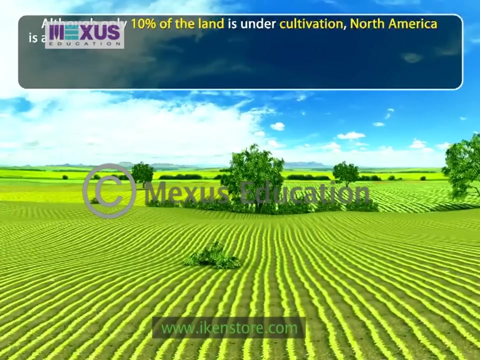 Mexico and countries of Central America have a large population. Mexico has tropical forests. Mahogany, logwood and cedar are important trees. of the tropical forests, These are called hardwood trees, Although only 10% of the land is under cultivation, North America is a surplus food producer. 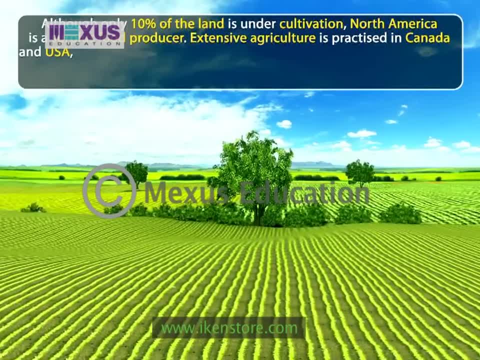 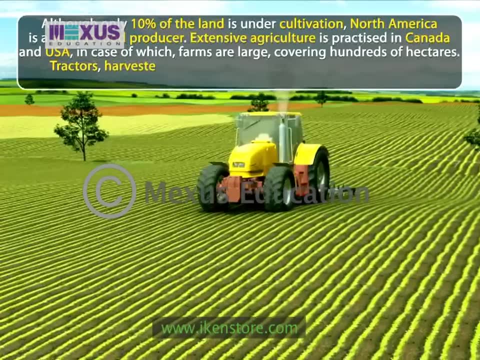 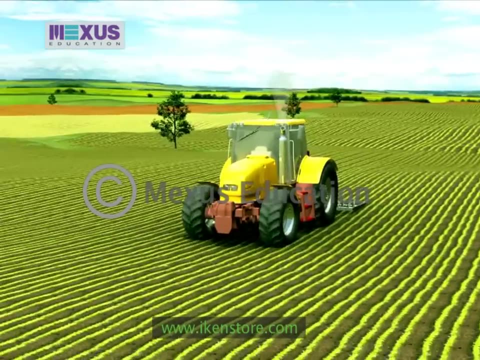 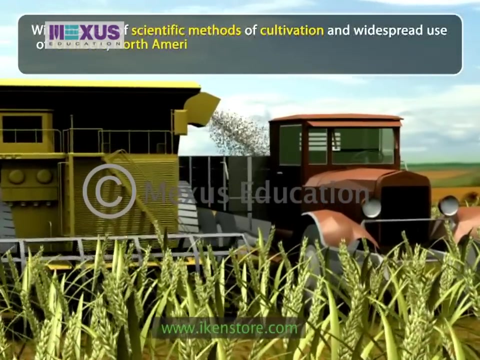 Extensive agriculture is practiced in Canada and USA, In case of which farms are large Covering hundreds of hectares. Tractors, harvesters and other machines are used for plying and other work on the farm, With the help of scientific methods of cultivation and widespread use of fertilizers. North America is the world's largest producer of maize, wheat and soybeans. 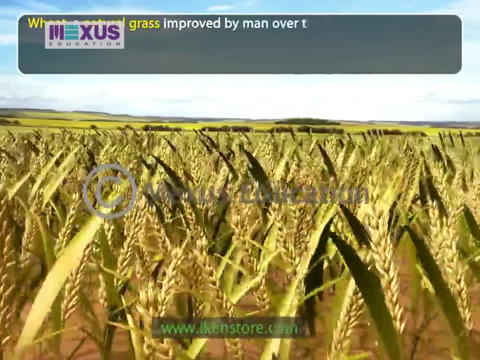 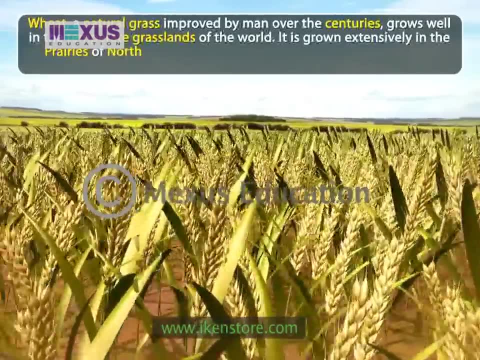 Wheat, a natural grass improved by man over the years, is the largest producer of maize wheat and soybeans. the centuries grows well in the temperate grasslands of the world. It is grown extensively in the prairies of North America where the soil is quite fertile and deep. Hence North. 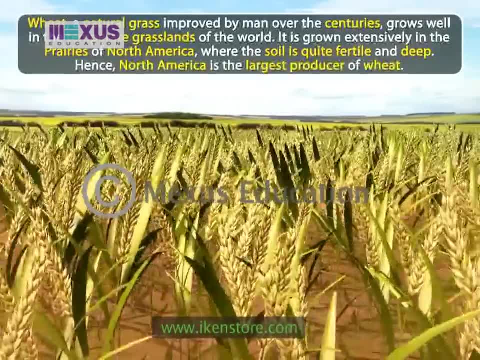 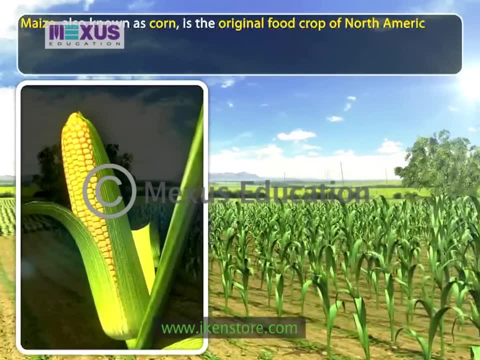 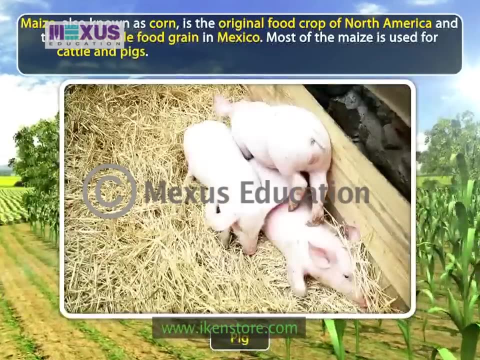 America is the largest producer of wheat. Maize, also known as corn, is the original food crop of North America and the main staple food grain in Mexico. Most of the maize is used for cattle and pigs. It is grown in large quantities in the southern prairies. as it 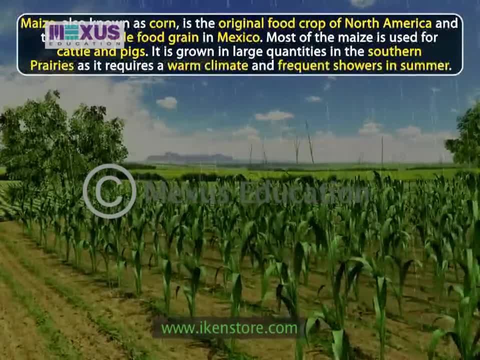 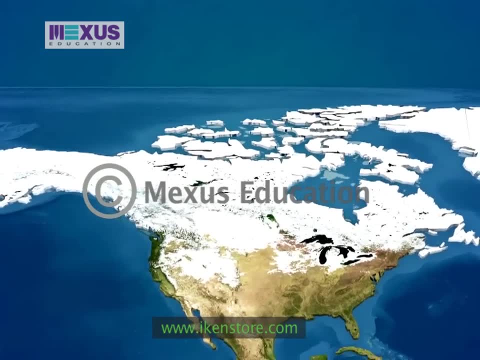 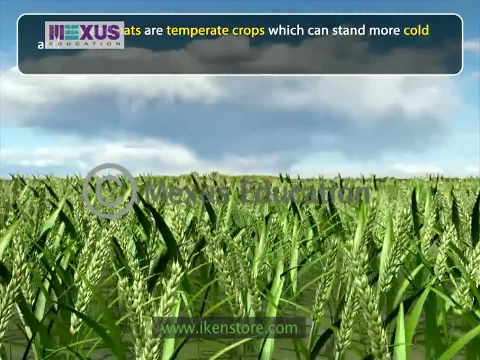 requires a warm climate and frequent showers in summer. North America produces more than half of the total maize produced in the world. Barley and oats are temperate crops which can stand more cold and need less water. Barley is used to make beer in large quantities. 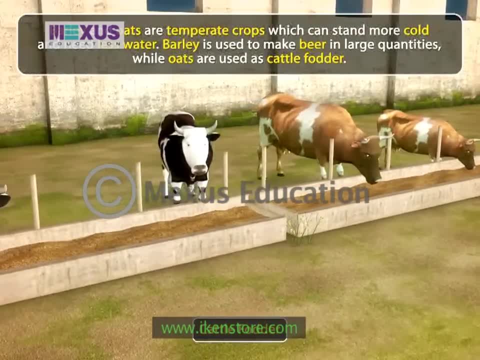 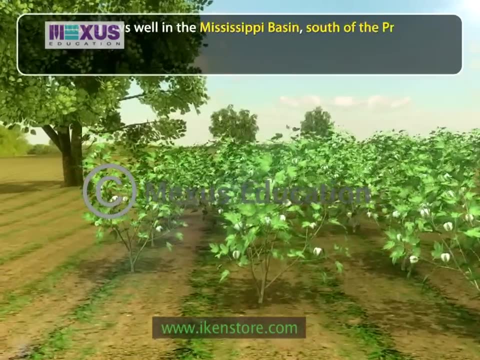 while maize is used to make beer in large quantities. Barley is used to make beer in large quantities, while maize is used to make beer in large quantities, While oats are used as cattle fodder. Cotton grows well in the Mississippi basin, south of the prairies, as well as in Mexico. 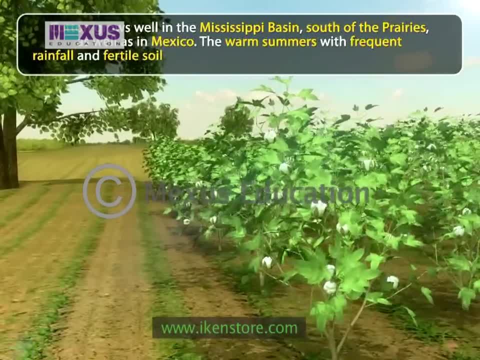 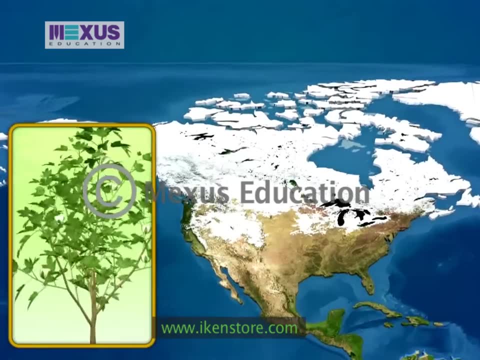 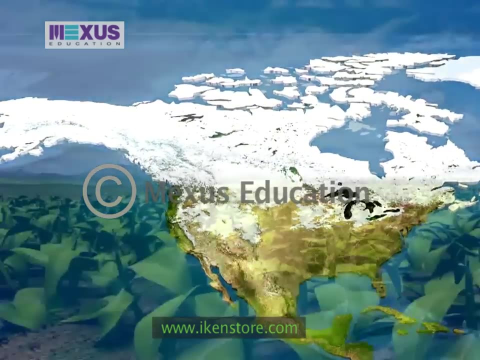 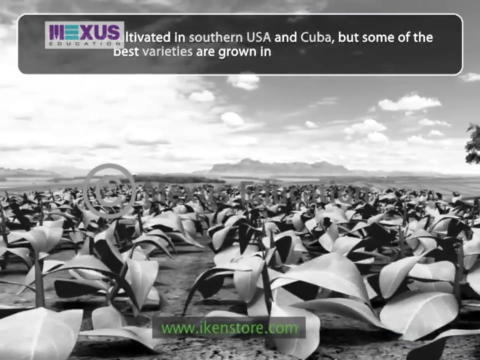 The warm summers with frequent rainfall and fertile soil provide suitable conditions for growing cotton. North America is the largest producer of cotton in the world and also produces the superior long staple variety. Tobacco is cultivated in southern USA and Cuba, but some of the best varieties are grown 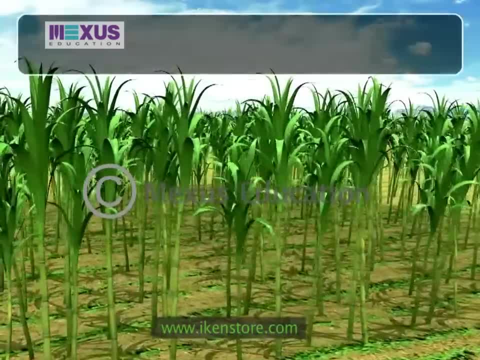 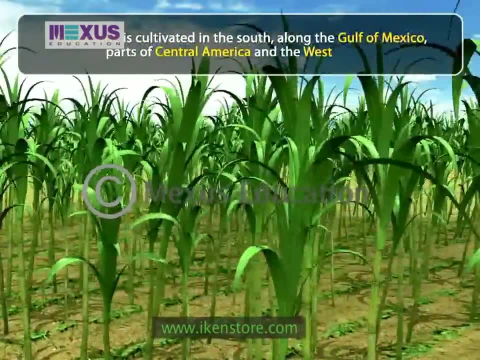 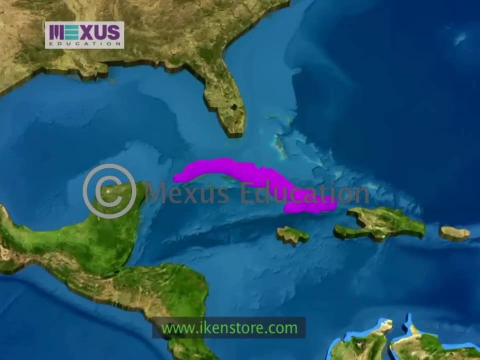 in North America. Sugarcane is cultivated in the south, along the Gulf of Mexico, parts of Central America and the West Indies. Cuba, known as the sugar bowl of the world, is the world's largest exporter of sugar. Soybean is an important crop in the United States. 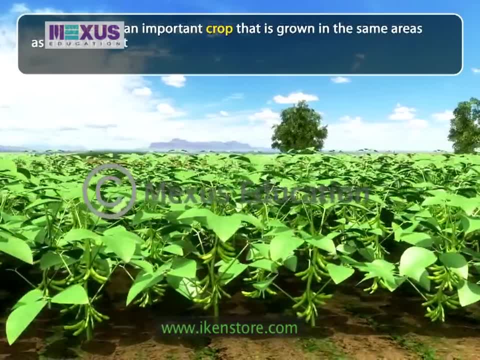 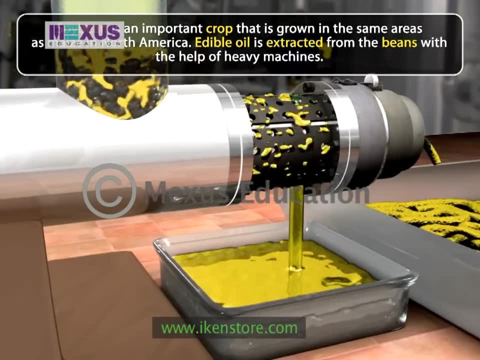 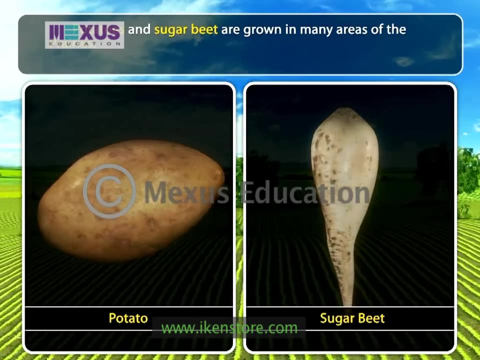 which is grown in the same areas as maize in North America. Edible oil is extracted from the beans with the help of heavy machines. Potatoes and sugar beet are grown in many areas of the prairies. Sugar beet is used for making sugar. Both the crops are used to feed cattle. 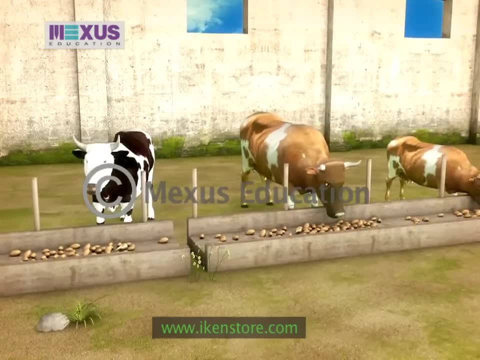 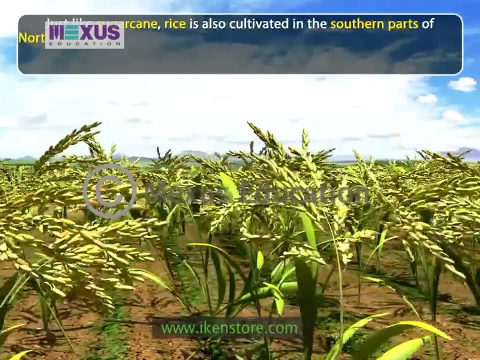 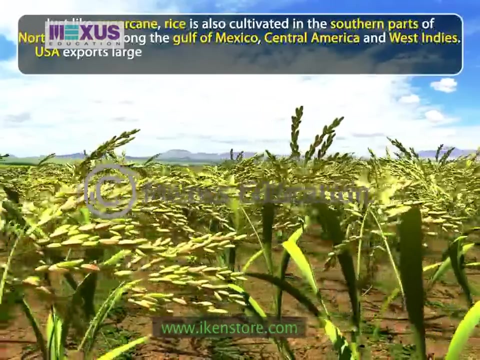 and pigs. Just like sugarcane, sugarcane is also used to make sugar. Sugarcane is used to make rice. Rice is also cultivated in the southern parts of North America, along the Gulf of Mexico, Central America and West Indies. USA exports large quantities of rice. 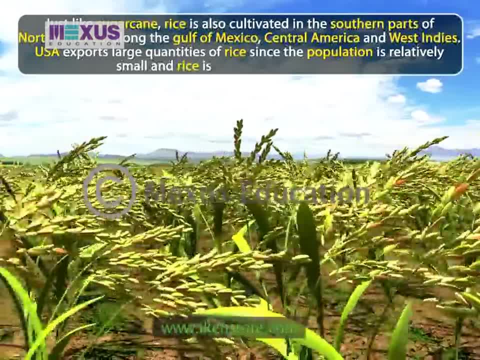 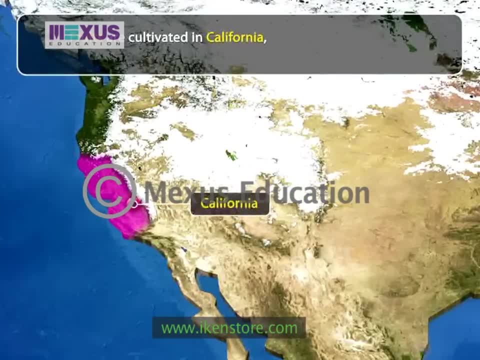 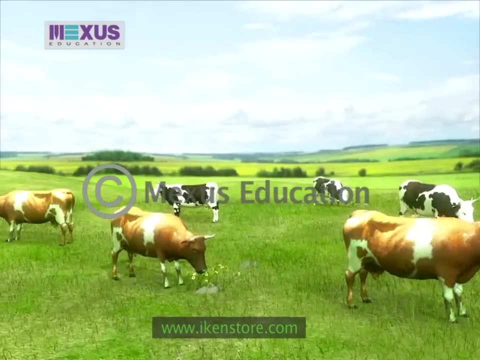 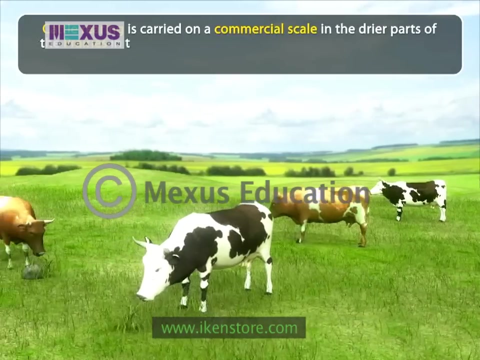 since the population is relatively small and rice is not the staple food here, Fruits are cultivated in California around the Great Lakes and the St Lawrence Valley. Cattle rearing is carried on a commercial scale in the drier parts of the prairies in. 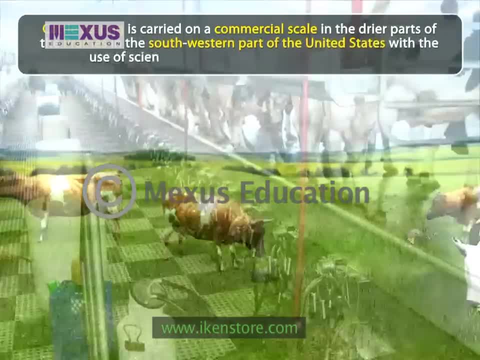 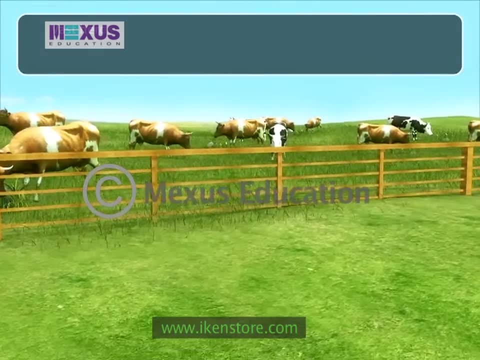 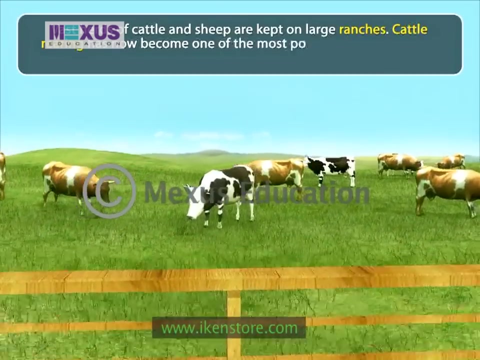 the southwestern parts of the United States, with the use of scientific methods and modern technology. Vast herds of cattle and sheep are kept on large ranches. Cattle rearing has now become one of the most popular industries in the country, considering its usefulness. 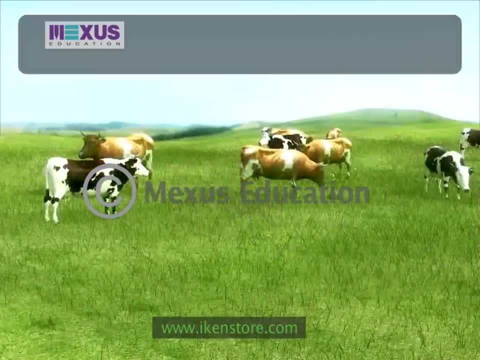 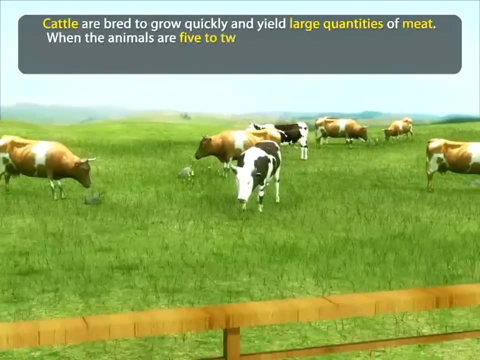 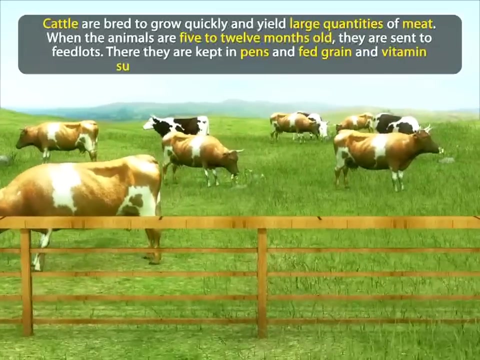 as well as revenue. Cattle are bred to grow quickly and yield large quantities of meat. When the animals are 5 to 12 months old, they are sent to feedlots. There they are kept in pens and fed grain and vitamin supplements until they reach market size. North America. 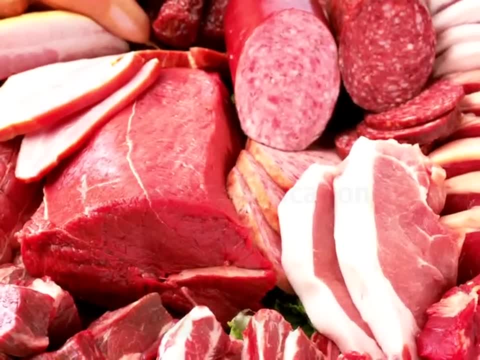 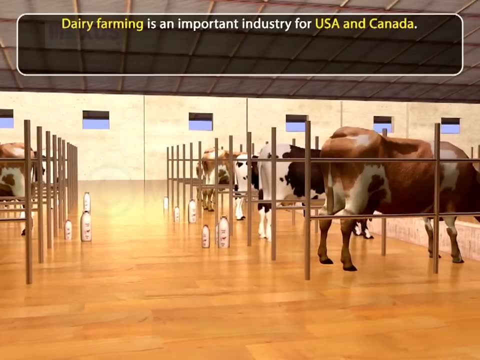 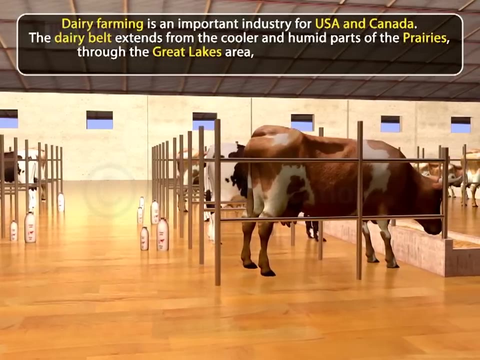 is the largest producer of meat, with about one-fourth of the world's production. Dairy selling is an important industry for USA and Canada. The dairy belt extends from the cooler and humid parts of the prairies through the Great Lakes area to the northeast region. 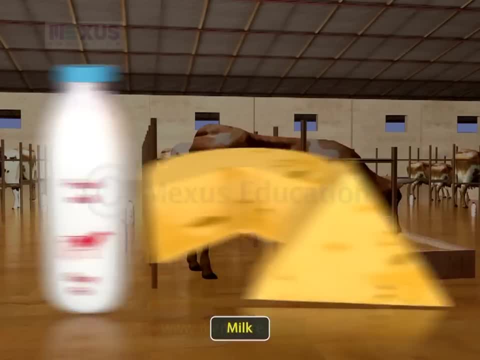 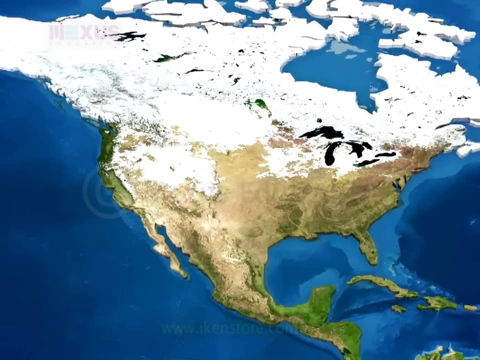 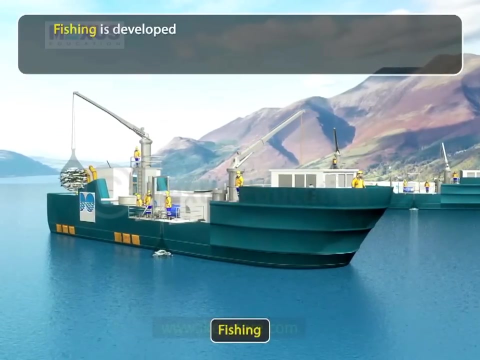 along the Atlantic coast. Milk, cheese and butter are the chief products. North America produces about 25 percent of the world's total milk and dairy products. Fishing is developed on a commercial scale in the seas around the continent. Grand Banks, one of the world's 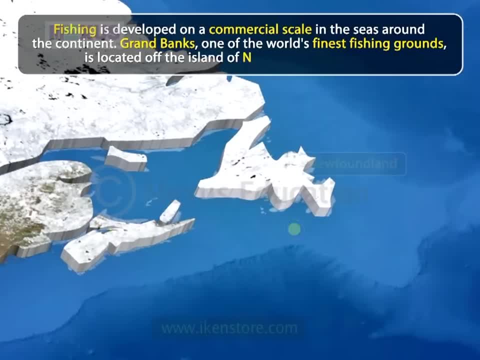 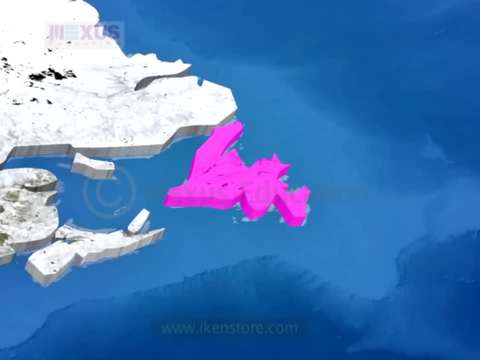 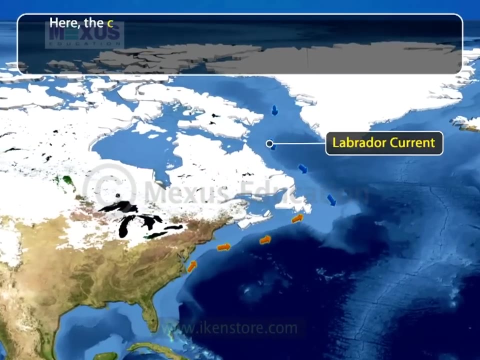 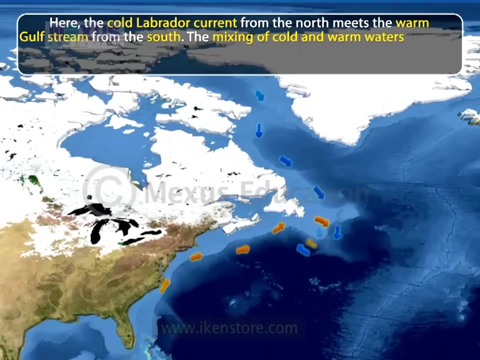 finest fishing grounds is located off the island of Newfoundland in Canada. It has an extensive continental shelf, making the water shallow enough for the sunlight to reach the bottom. Here the cold Labrador current from the north meets the warm Gulf Stream from the south. The mixing of cold and warm waters provides the best quality of life for the 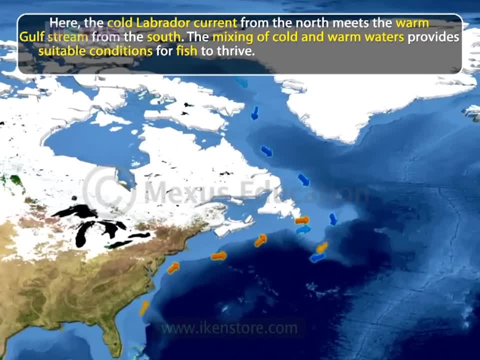 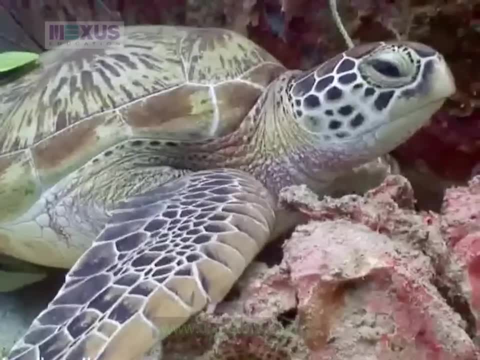 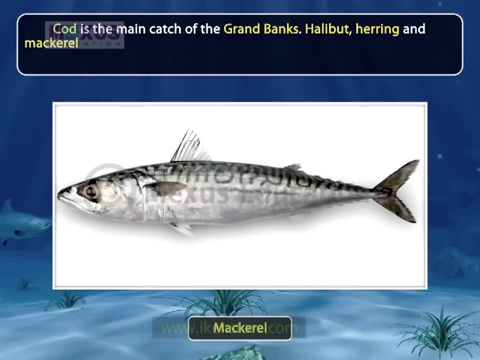 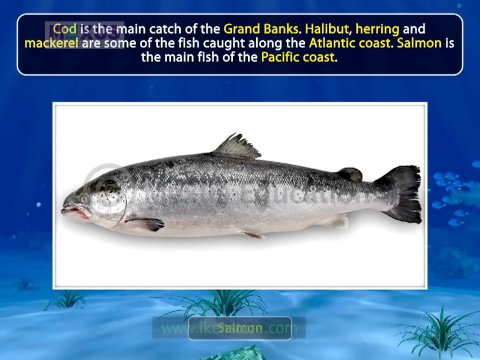 fish. The cold Labrador current also brings plenty of plankton, which provides food for fish. Cod is the main catch of the Grand Banks. Halibut, herring and mackerel are some of the fish caught along the Atlantic coast. Salmon is the main fish of the Pacific coast. 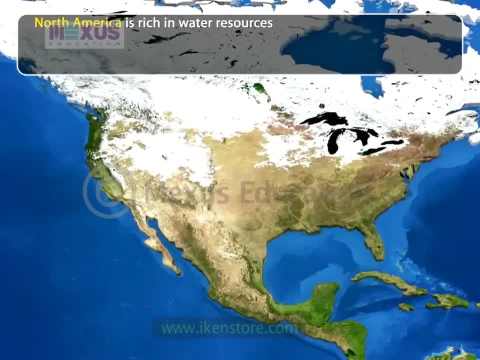 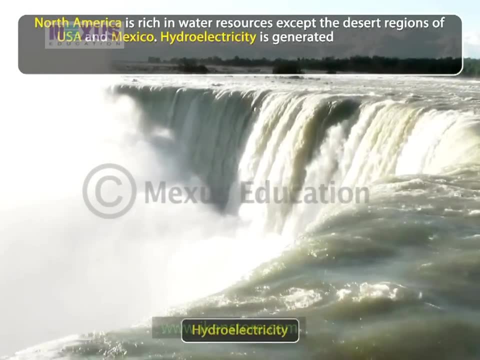 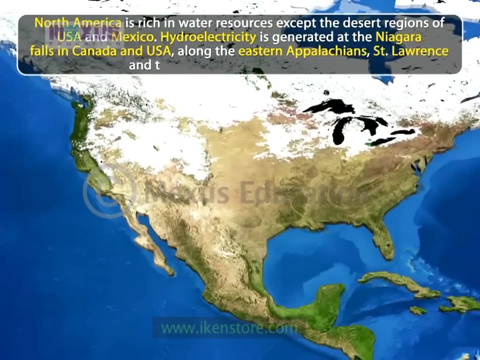 North America is rich in water resources, except the desert regions of USA and Mexico. Hydroelectricity is generated at the Niagara Falls in Canada and USA, along the eastern Appalachians, St Lawrence and the rivers of the Canadian Shield. North America is now. 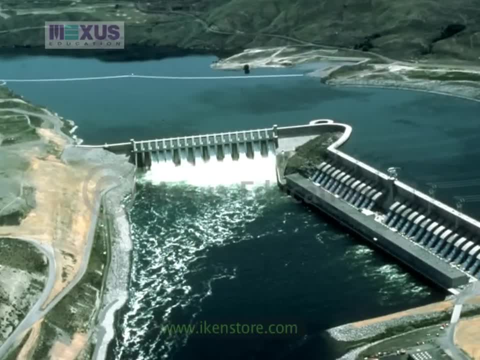 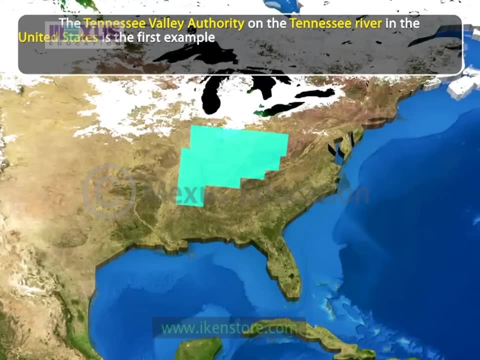 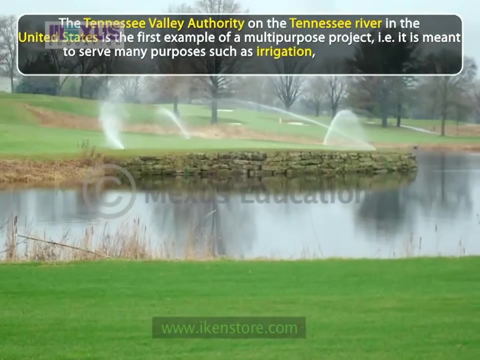 the largest producer of hydroelectricity. The Tennessee Valley Authority of the Tennessee River in the United States is the first example of a multi-purpose project, That is, it is meant to serve many purposes, such as irrigation, hydroelectricity, flood control and navigation.